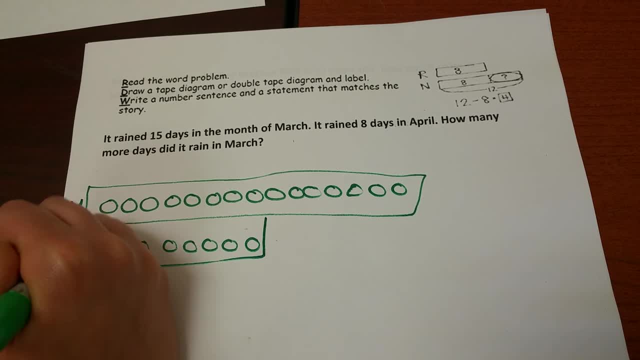 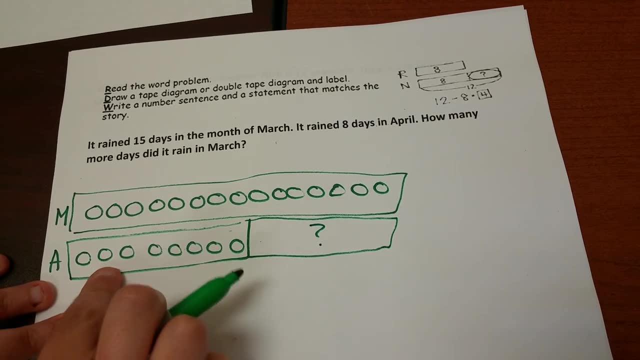 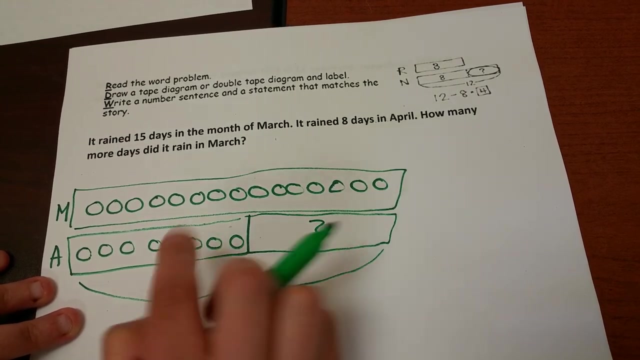 25,, 26,, 27,, 28.. 8 days in April. The problem is asking: how many more days did it rain in April than March? Knowing that my total is going to be 15, I have 8 here for April. How? 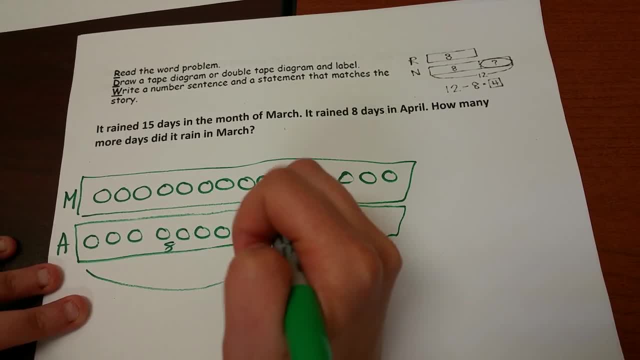 many more do I need To figure it out? I'm going to travel my line up so I can compare them. If this is the 8th, I'll need 1,, 2,, 3,, 4,, 5,, 6,, 7,, 8,, 9,, 10,, 12,, 13,, 18,, 19,, 20,, 21,, 21,. 22,, 23,, 24,, 25.. If this is the 8th, I'll need 1,, 2,, 3,, 4,, 5,, 6,, 7,, 8.. If this is the 8th, I'll need: 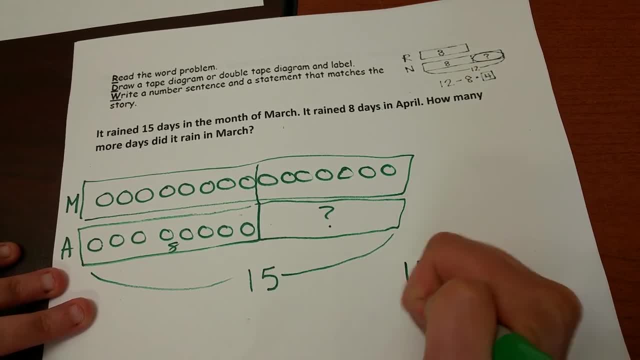 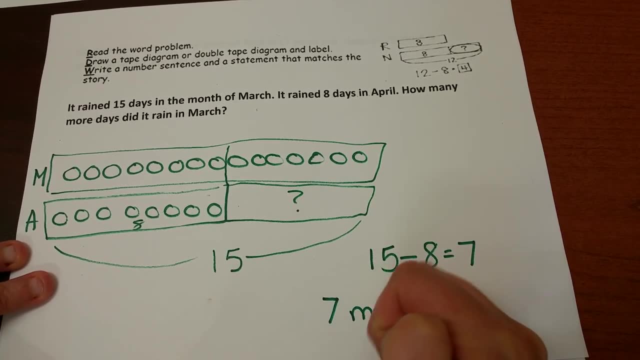 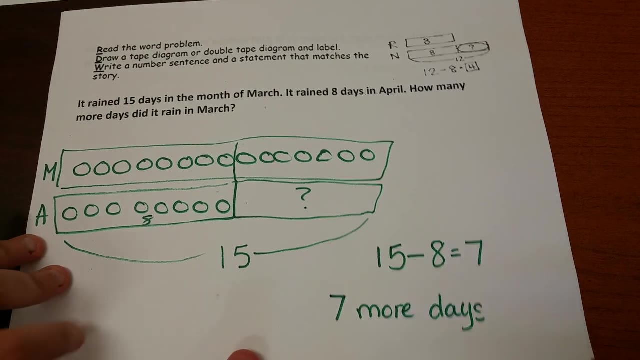 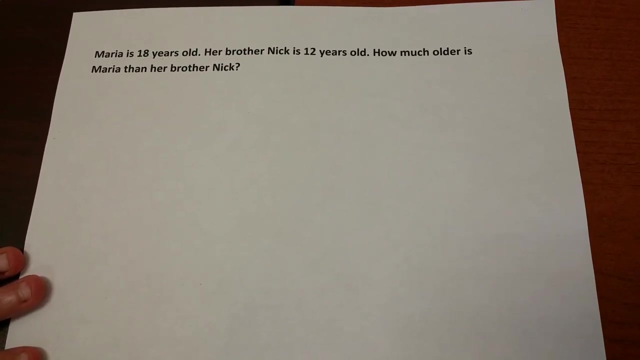 three, four, five, six, seven. Fifteen minus eight equals seven. There are seven more days in March. Let's do it one more time. Maria is 18 years old. Her brother, Nick, is 12 years old. How much older is Maria than her brother? 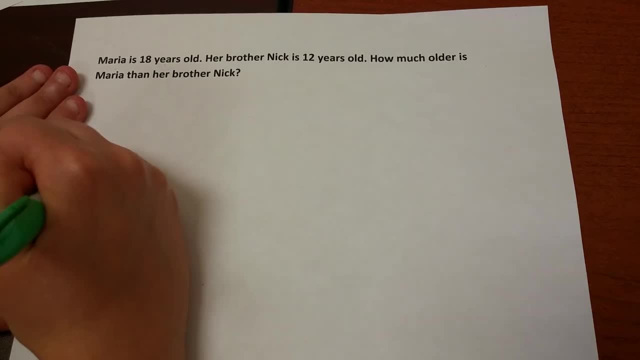 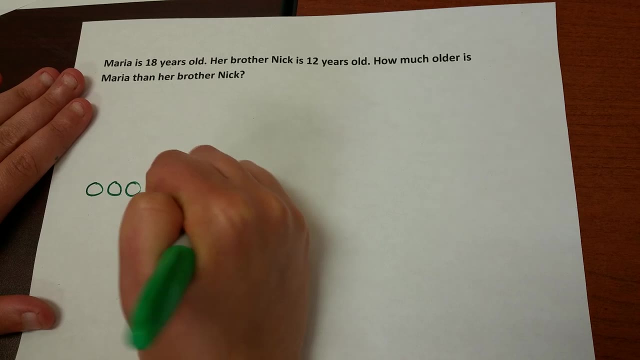 Nick, If I wanted to do it with a single tape diagram, it's the same basic concept. I would start with the first number: Maria is 18.. Two, three, four, five, six, seven, eight, nine, ten. 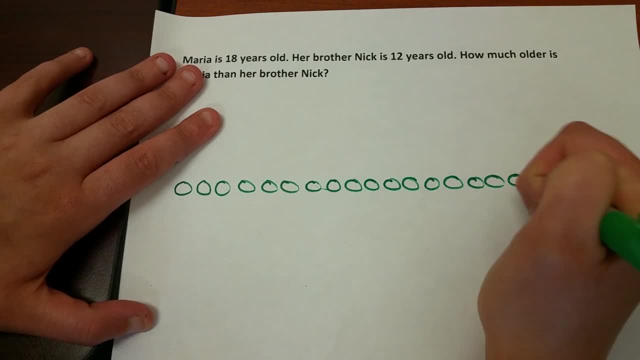 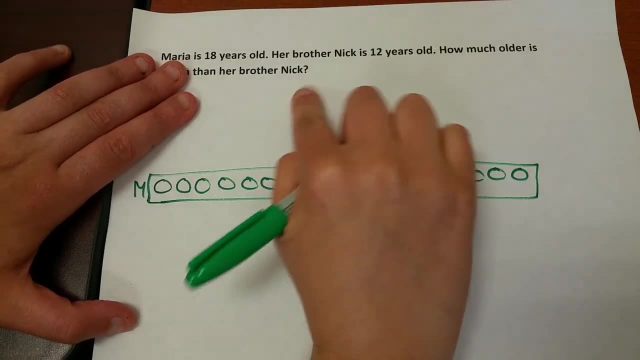 eleven, twelve, thirteen, fourteen, fifteen, sixteen, seventeen, eighteen. That's Maria, And I want to know how much older she is. Her brother, Nick, is 12.. So instead of drawing a second tape diagram, I can just cut it in half. 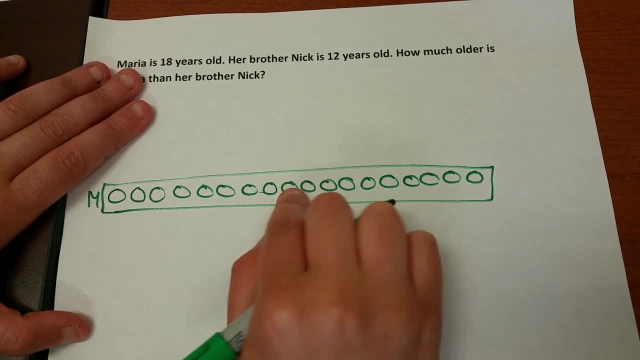 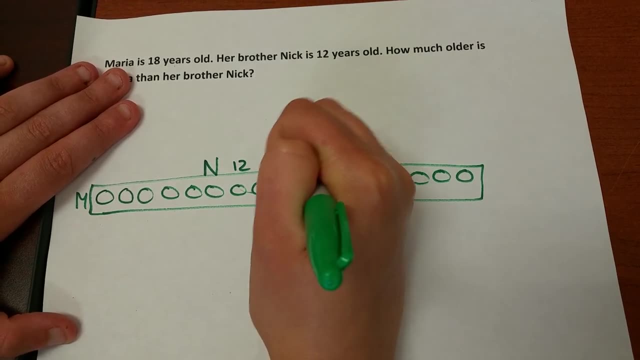 So let's get where the 12 is: One, two, three, four, five, six, seven, eight, nine, ten, eleven, twelve. This is Nick He's 12. And this is how much older she is. So the total is Maria's. 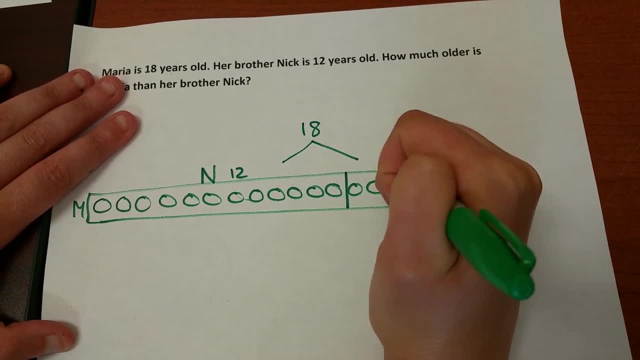 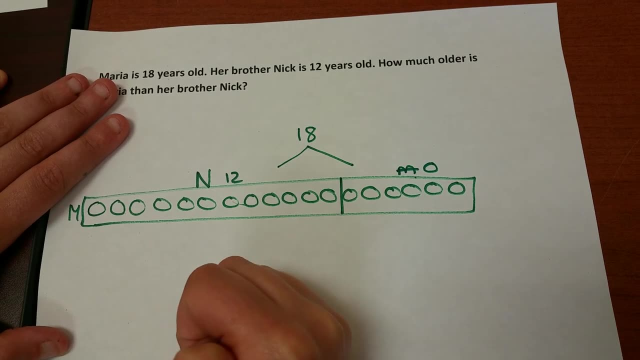 18.. One, two, three, four, five, six. This is how much older she is, How many more years she has. Older probably would be a better label. So we had 18.. We took away the 12. Our 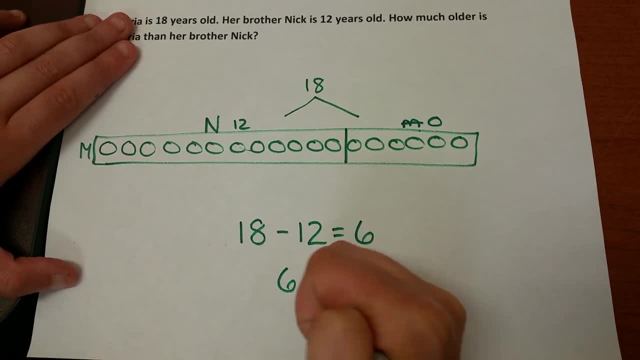 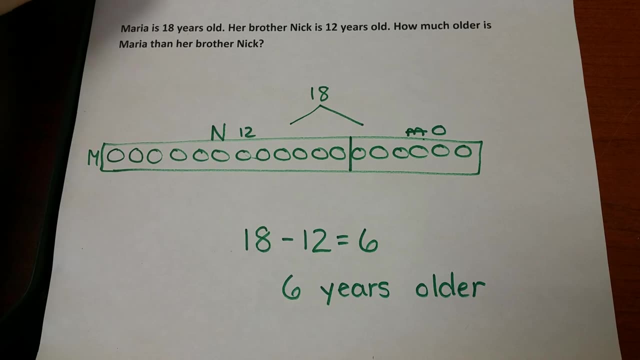 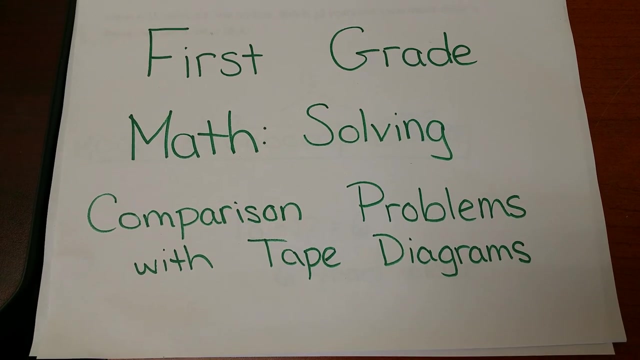 answer is 6.. She is six years older. That's how you use tape diagrams to compare in first grade. Thank you very much for watching.